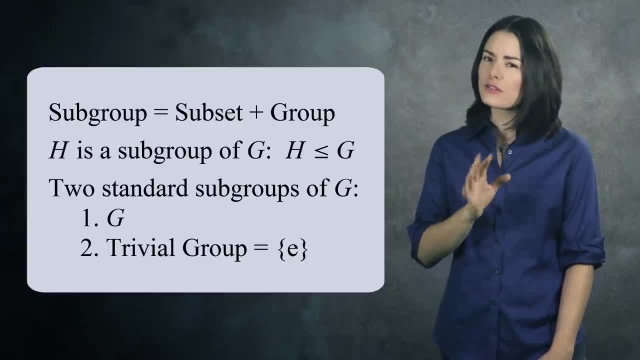 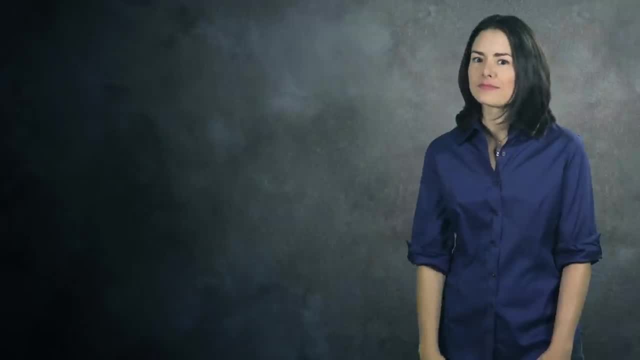 But these subgroups are fairly dull. We want to see if G has a subgroup other than these two. Something more interesting. 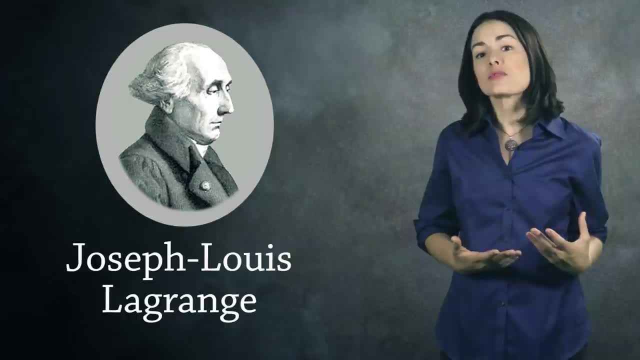 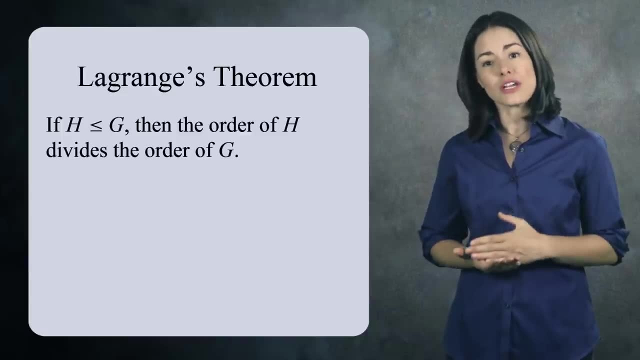 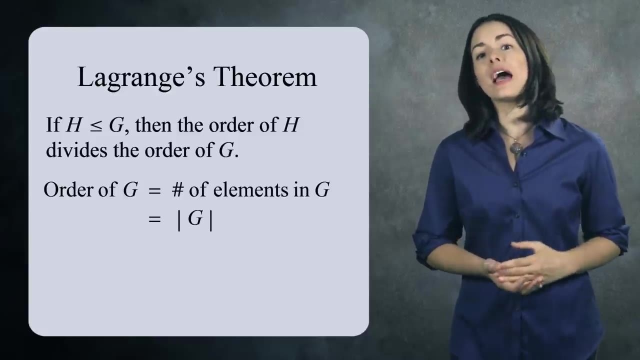 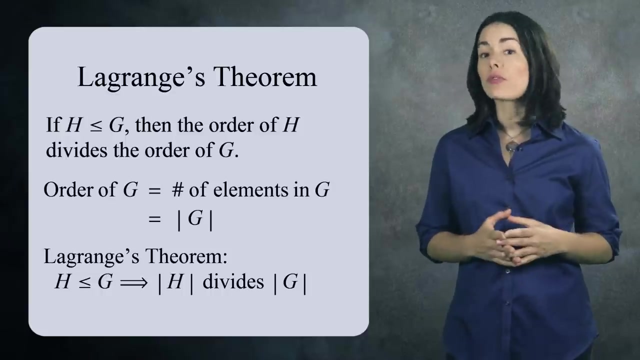 The mathematician Joseph-Louis Lagrange found a useful test which we now call Lagrange's theorem. He discovered that if H is a subgroup of a finite group G, then the order of H divides the order of G. Recall that the order of a group is a number of elements in the group, and it's denoted by the absolute value symbol. With this notation, we can write Lagrange's theorem more compactly. This is a powerful result. It says that subgroups can't be any old size. There are strong restrictions on the possible subgroups of G. 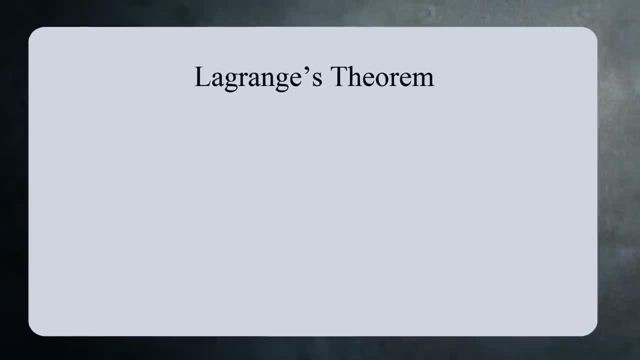 Before proving this theorem, let's see just how useful this is. Imagine you have a group G with 323 elements. You can factor this as 17 times 19. This means the only positive integers dividing 323 are 1, 17, 19, 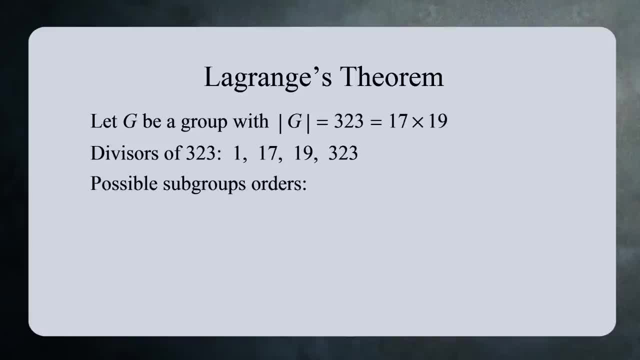 and 323. So any subgroup of G must have order 1, 17, 19 or 323. Earlier we mentioned that every group has at least two subgroups, itself and the trivial group. The group itself has order 323, and the trivial group has order 1. This means 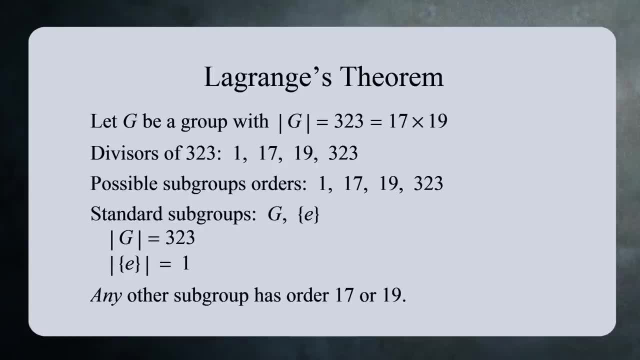 if G has any other subgroups, their orders are 17 or 19. has shortened dramatically. 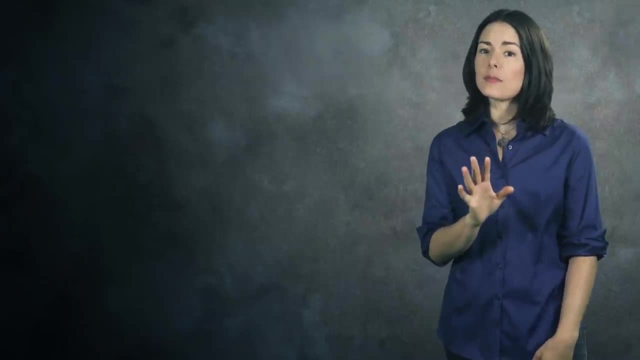 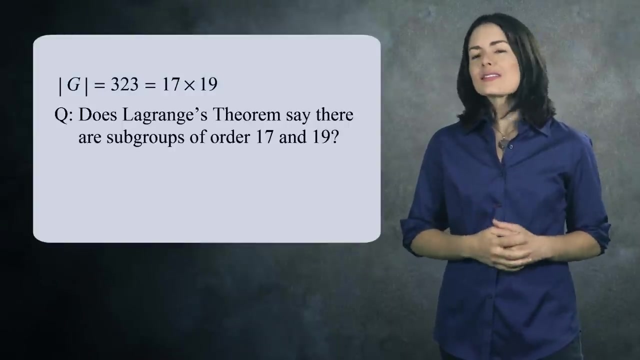 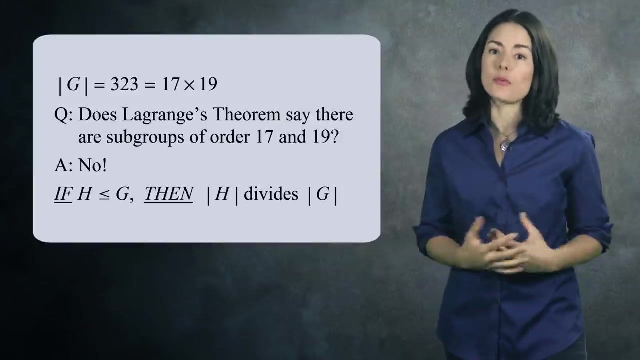 This is a good moment to pause and not get overly excited about Lagrange's theorem. We need to learn its limitations. 17 and 19 divide the order of G. Does Lagrange's theorem say that there are subgroups of these orders? No. Lagrange's theorem is an if-then theorem, which means the converse may not be true. 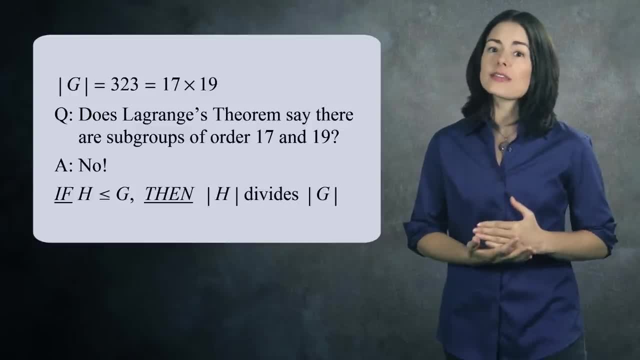 Just because a number divides the order of G, there's no guarantee that a subgroup of this size will exist. 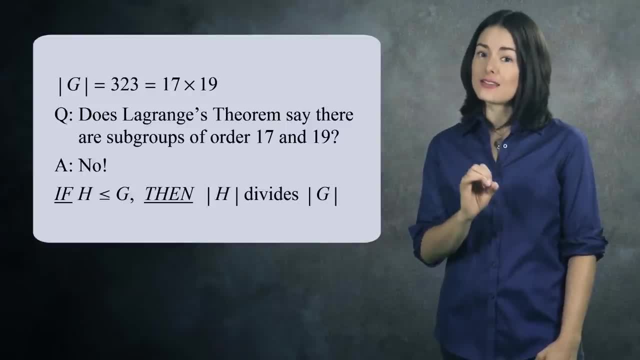 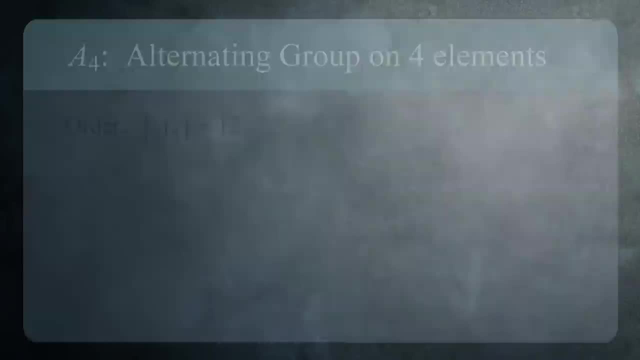 In this case, it just so happens that G does have subgroups of orders 17 and 19, but there are groups where this isn't the case. 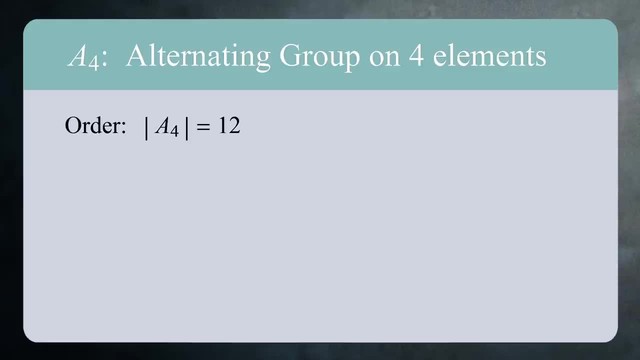 For example, there's a group with 12 elements called A4, the alternating group on 4 elements. The divisors of 12 are 1, 2, 3, 4, 6, and 12, so any subgroup must have one of these orders. However, even though the number 6 divides 12, this group does not have a subgroup of order 6. 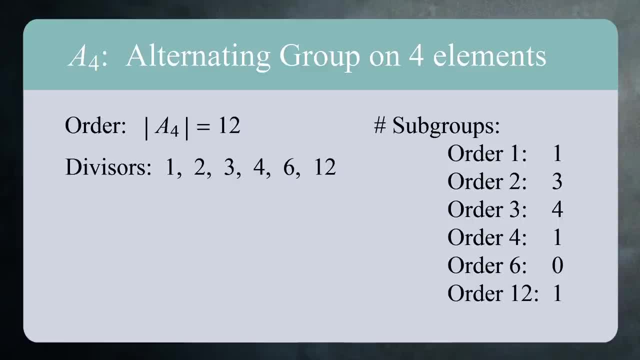 But it does have subgroups of the other possible orders. This is a cautionary tale on the limitation of Lagrange's theorem. 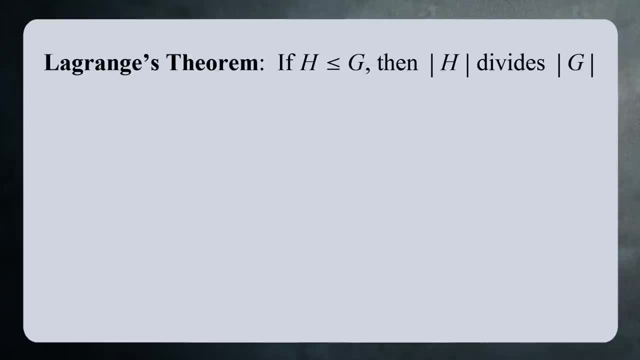 Let's now roll up our sleeves and get to work proving this theorem. 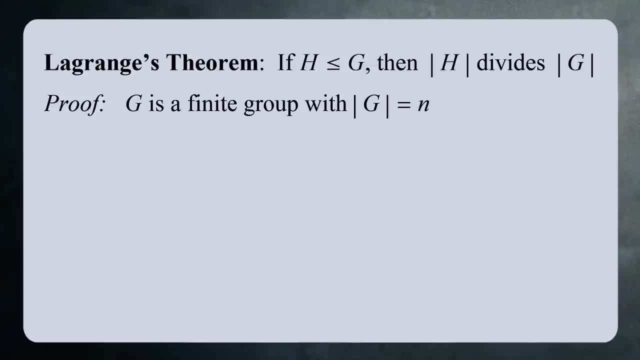 Suppose we have a random finite group G with order n. To start, let's check the two easy cases of the trivial group and the group itself. The trivial subgroup has order 1, and 1 divides n. Next, the group itself has order 2. The trivial subgroup has order 1, and 1 divides n. The group itself has order n, and n divides n. So Lagrange's theorem works for both of these cases. 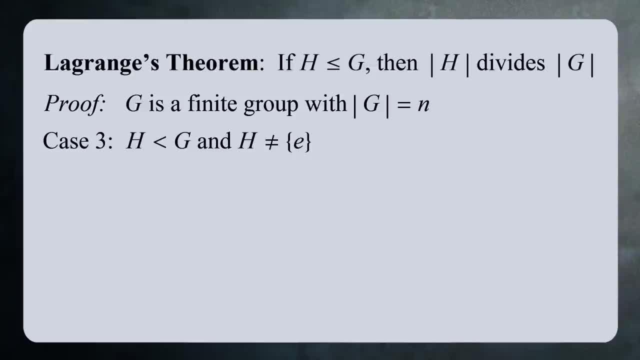 Now suppose that G has a proper subgroup H that's NOT the trivial group. Recall that a proper subgroup is just a subgroup that's smaller than G, one that's a proper subset. 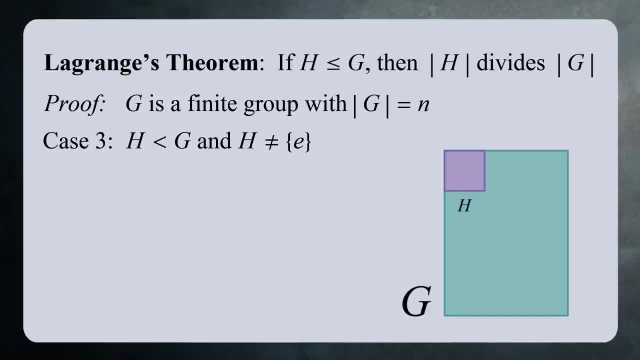 We'll represent the group G by a rectangle, and H as a small square inside G. Because H is a group, it contains the identity element. So the identity element for both G and H lies inside G. If we divide by H, the suitability of g and h is automatically hurtord, WE MAKE THIS TECHNIQUE PRIME! !. There is no super important idea here. You can break the set in any household by analyzing the less important parts of it and 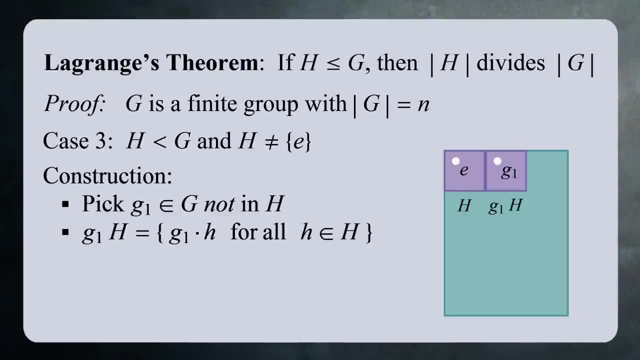 Jacob is going to make a simple math project by the tool D 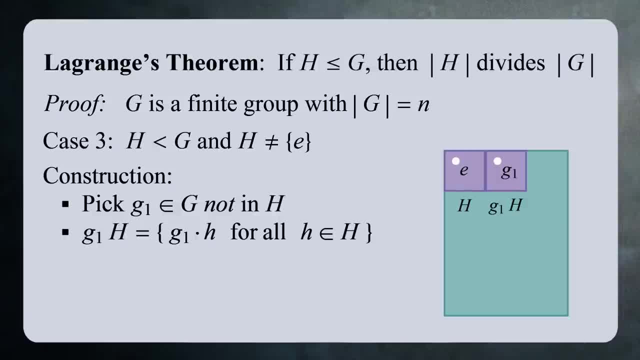 and the answer is c Literally half destroying a big pile of Carl'sавно Wenn מה How did Einstein finish out the test on seeing how long a косet could last? We can draw one 1930-thousand-year-old thinlong tongue, let's say 100 meters long, from a иф- scenery and weigh in here. D is divided by h. 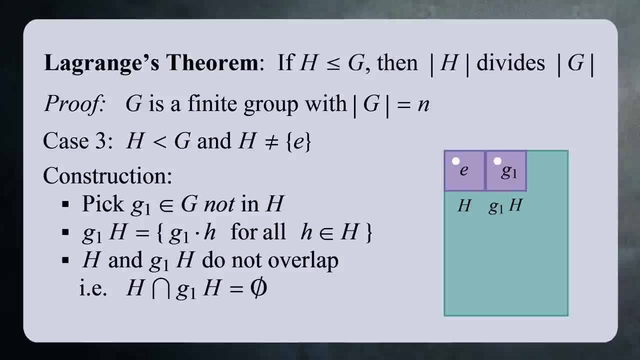 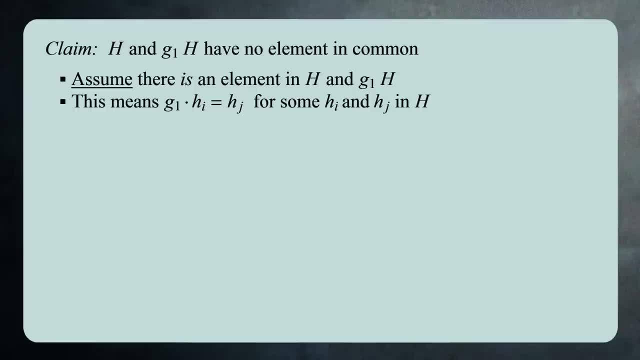 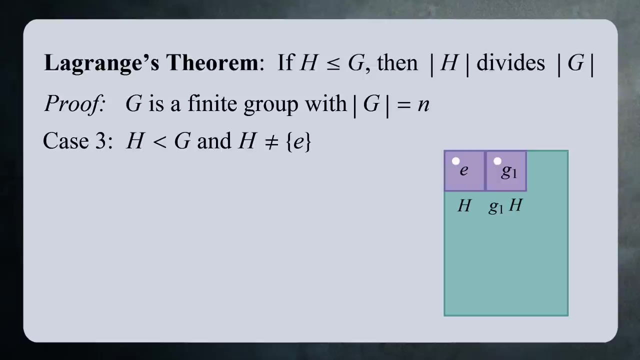 in common. Their intersection is the empty set. Here's why. Let's assume that there is an element in both H and G1H. This means G1 times HI would equal HJ for some elements HI and HJ in the subgroup H. If you multiply this equation on the right by the inverse of HI, then simplify, you get G1 equals HJ times HI inverse. Since H is a subgroup, the right-hand side is in H, so G1 is in H. But this is a contradiction. We specifically chose G1 to NOT be in H. So our assumption must be wrong, and the two sets do not overlap. We're going to repeat this process until we get to the point there's no element in G that's not in a coset. Pick an element G2 that lies outside both H and G1H. Again, we'll look at the left coset G1H. 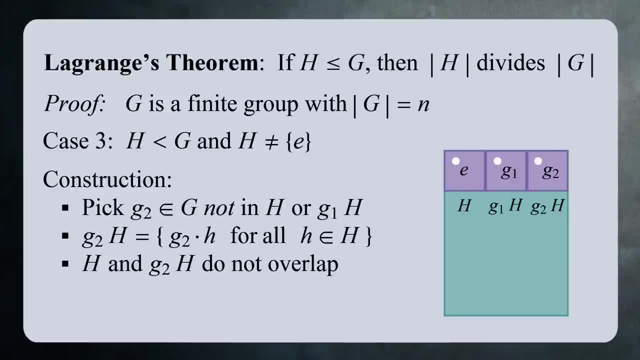 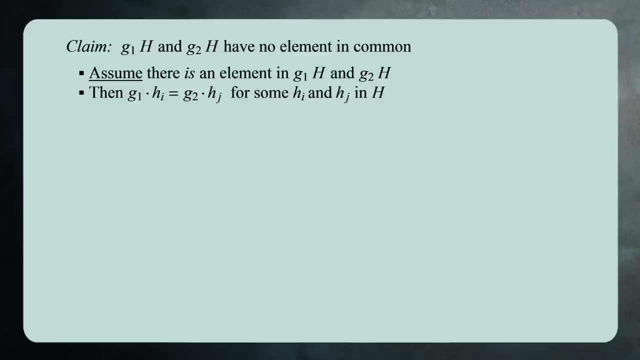 Using the same argument as before, H and G2H do NOT overlap. Next, we'll show that G1H and G2H do not overlap either. Assume they DO overlap. Then G1HI equals G2HJ for some elements HI and HJ in the subgroup H. If you multiply both on the right by HJ inverse, simplify, you get G1 HI HJ inverse equals G2. But HI equals G2. HI times HJ inverse is an H, call it HK, which means G1HK is in the left coset G1H. This means that G2 is in the coset G1H. But we specifically chose G2 to be OUTSIDE of G1H. So our assumption was wrong, and they do NOT overlap. 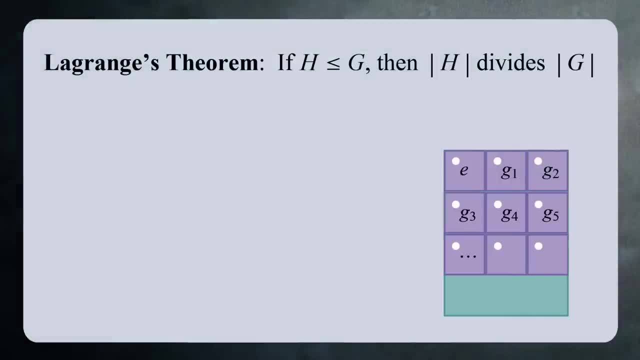 Continue this process until you get to the point that there's no element left that's not in a coset. The result is we have partitioned G into a collection of non-overlapping left cosets. 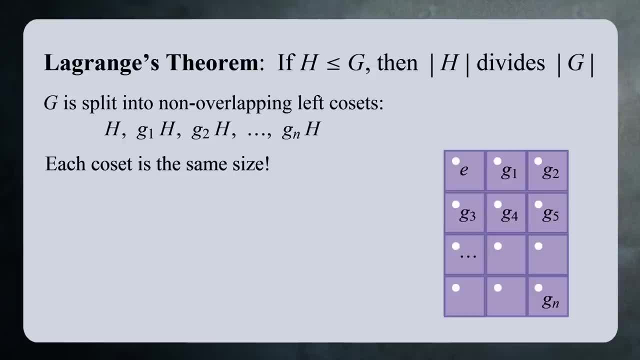 There is one more thing. All the cosets are the same size. There is a short proof for this. Consider a left coset GH. Suppose this set contains a duplicate element. This means GH1 equals GH2 for different elements H1 and H2. But if you multiply on the left by G inverse, you see that H1 equals H2. This means that the size of each left coset is equal to the order of H.